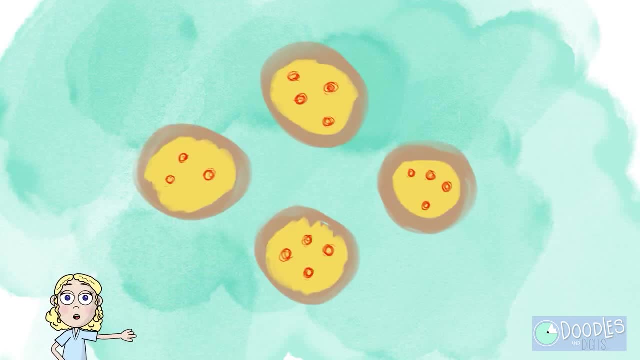 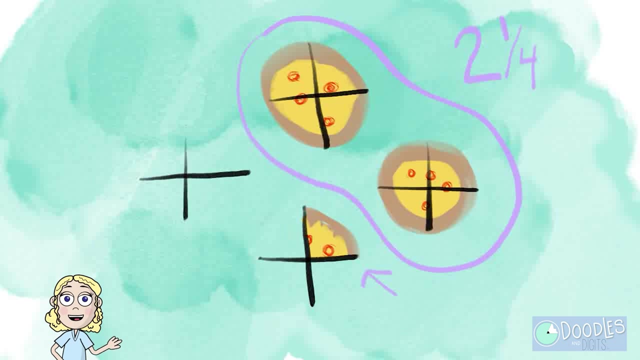 number. If you were having a pizza party, you wouldn't necessarily say the exact fraction of pizza left over. You would say the mixed number. It's easily understandable in conversation and you can quickly understand what's going on with the numbers. There's actually a couple. 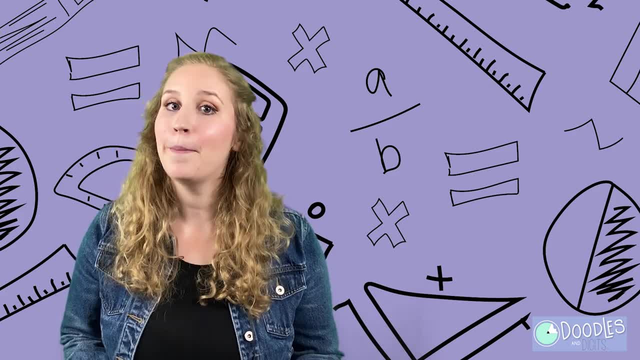 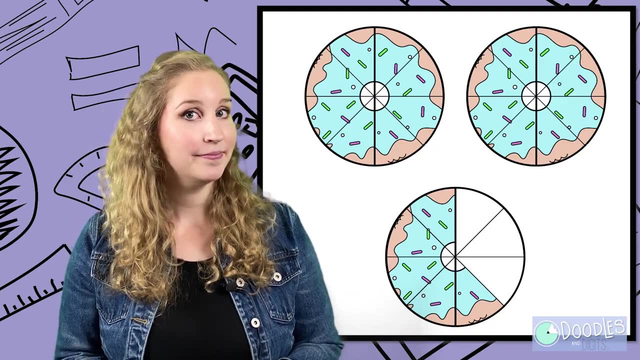 different ways that you can show a mixed number. Let's look at a couple models and see if you can figure out what mixed number I'm showing. All right, what mixed number is this? There are two whole donuts here, and then, when we look at the fraction, 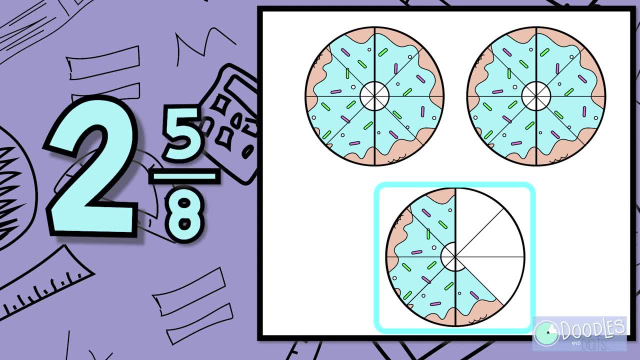 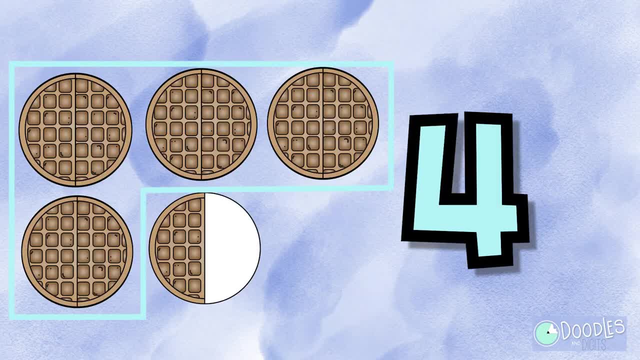 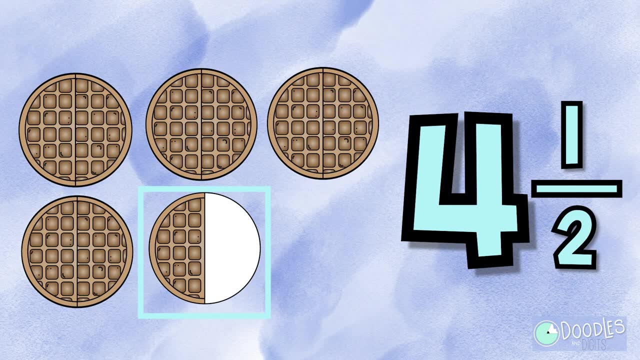 there's five out of the eight pieces left over, so our mixed number is two and five-eighths. Let's try another one. How about this? There are four whole waffles here, so our whole number is four. Then our fraction: there's one half of a waffle left over, so our mixed number is four, and 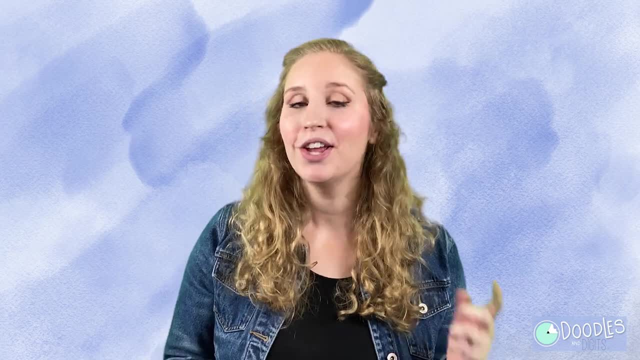 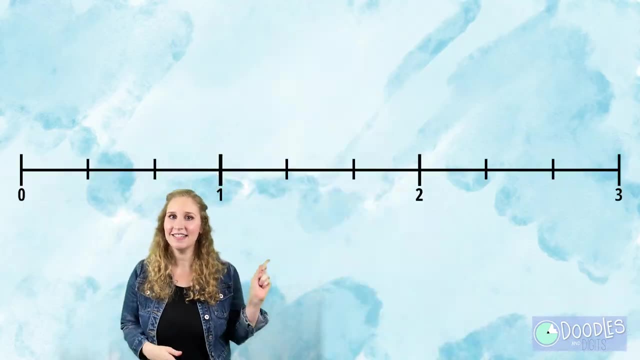 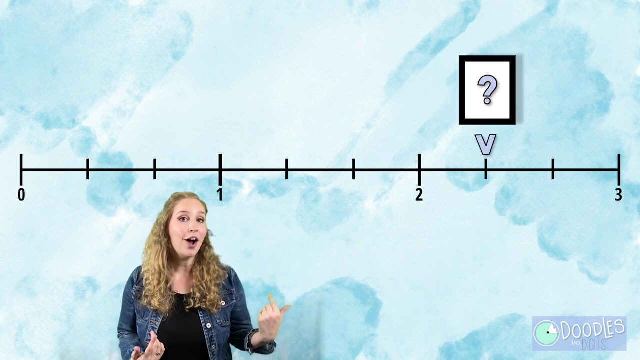 a half. Not only can you show mixed numbers with models, you can also use a number line. Let's try one now. Number line: All right, this number line right here is showing a mixed number. What mixed number do you think it's showing? You might notice, on this number line you have wholes and you also have fractions. 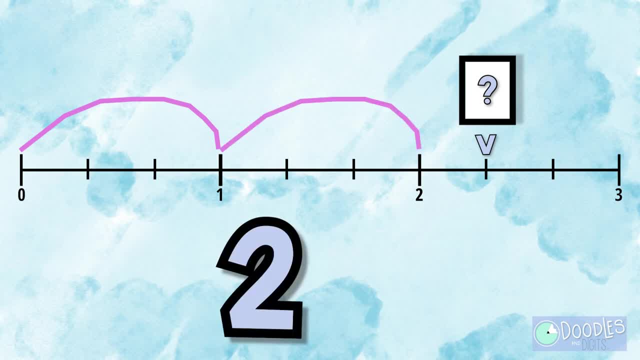 Let's first see how many whole numbers we're jumping. We're jumping two whole numbers, so our whole number is going to be two. Now we're going to look at the fraction and try to figure out what it's broken down into. It's broken down into thirds, so our denominator will be three. 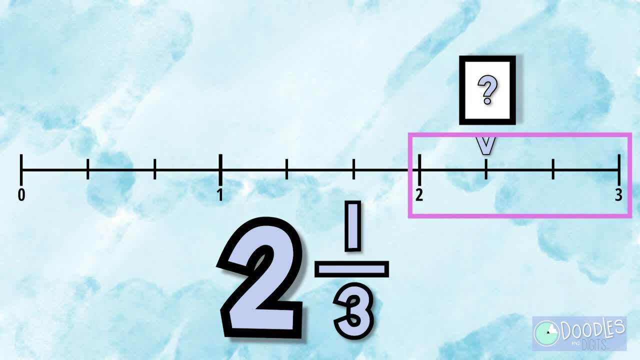 How many thirds we jump. We jump one-third after two, so our mixed number will be two and a third. Remember, you can take your time and double and triple check to make sure that you got the correct answer. All right, let's try a few more together. 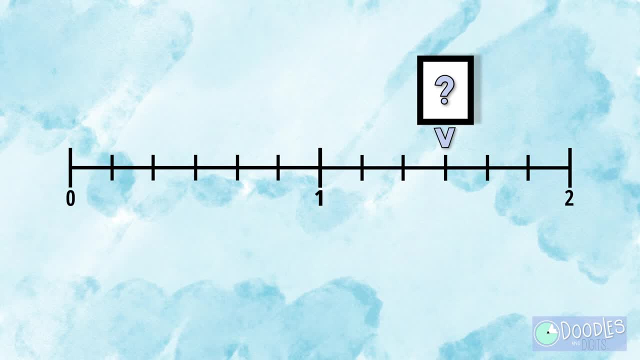 All right, what mixed number is this number line showing? Let's first do our whole number jump. so we have jumped one whole number. Now let's try to figure out what fraction number line is showing. It's broken down into sixths, so we're going to put six on the denominator.